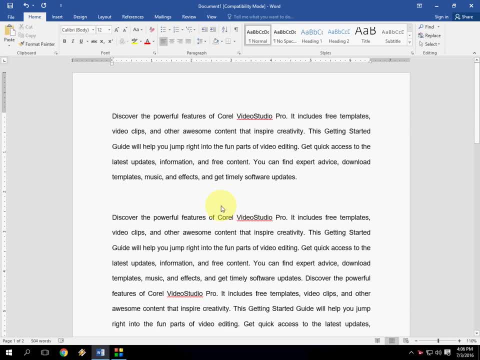 Welcome back again. I'm MJ. In this video I'll show you how to count word, paragraph lines etc. in Microsoft Word. So normally when you select the any text or word, it will show here in the bottom the page numbers and the word. 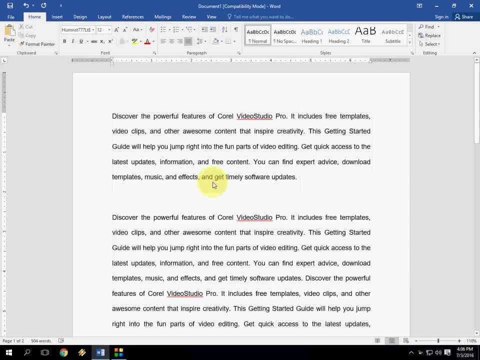 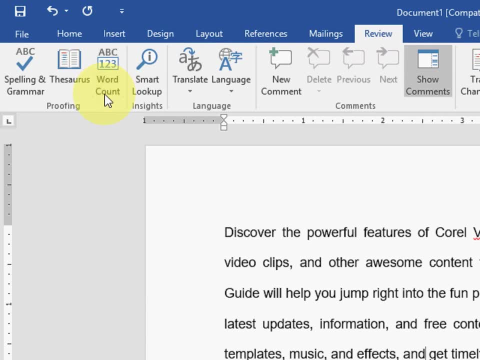 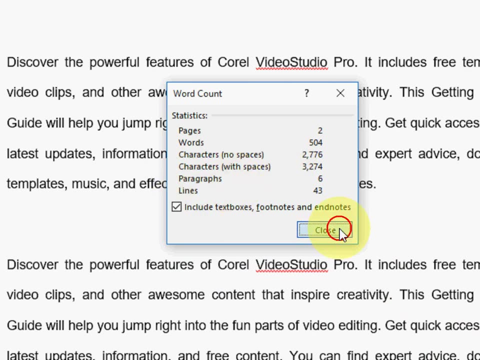 But if you want to go in detail, we need to click on review, then click on here what count. Then you will get the all detail about the pages, words, character, paragraph lines. But instead of doing this, you can use a simple keyboard shortcut key. 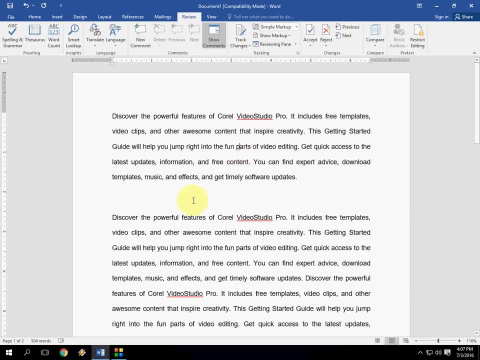 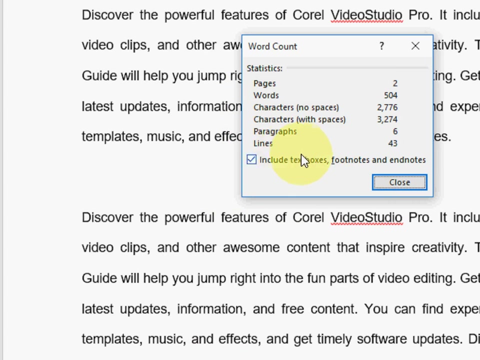 So the key is just open your any document and keep your cursor anywhere, Doesn't matter. Press control shift. Don't be confused about key. Hold control shift key and press G. Look at that. The same thing is up here, like pages, word, character and paragraph line. 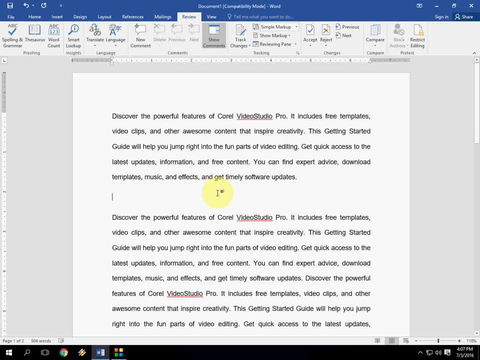 So again hold the control shift key and press G button to count your word, pages, paragraph lines, etc. in the Word document. So this is the keyboard shortcut key of checking your words, paragraph lines in MS Word And this key will work all the version of your Microsoft Word, like 2003,, 7,, 10, 2016.. 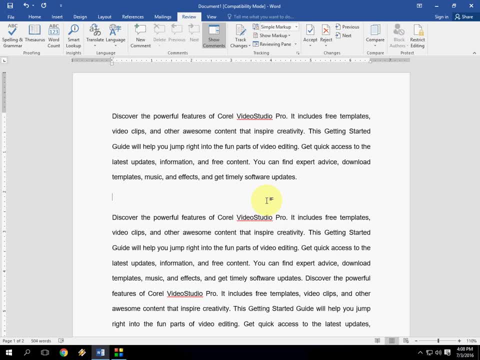 And yeah, that's it: 2016,. last version, I think. So that's it for today. Thanks for watching. See you in next video. Please like, share and subscribe. Thank you very much.